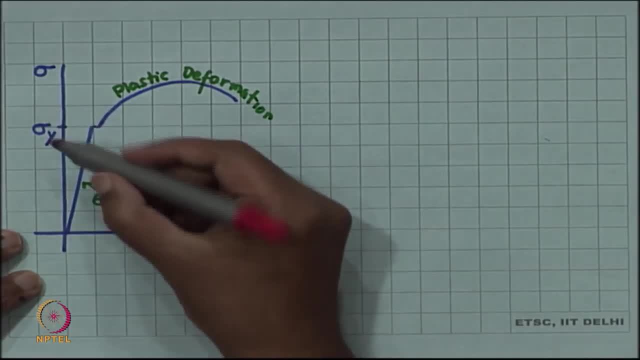 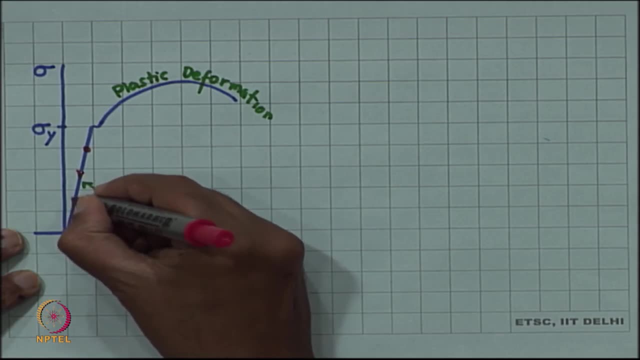 video. we saw the uniaxial tensile test and we saw that the initial part was in elastic deformation, but that was followed by plastic deformation. So if we start unloading at any point in the elastic part of the curve, then there will be no permanent deformation, but 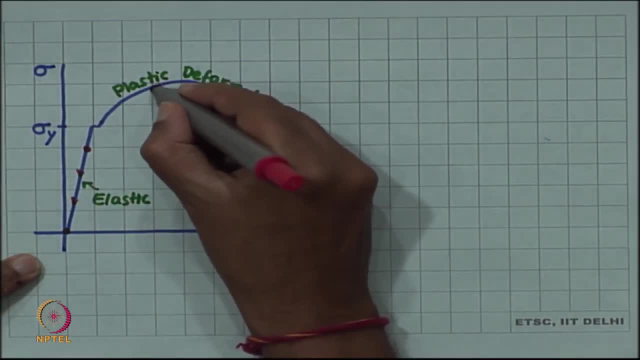 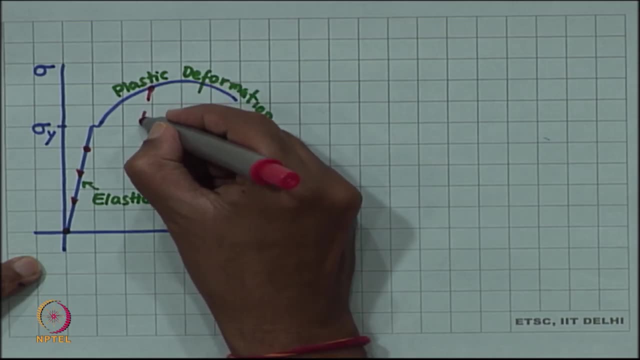 if we, after we have deformed, let us say, up to a certain point in the non-linear regime and from there if we unload, then it will follow a line. So let us continue our discussion of the mechanical behavior of materials In the last 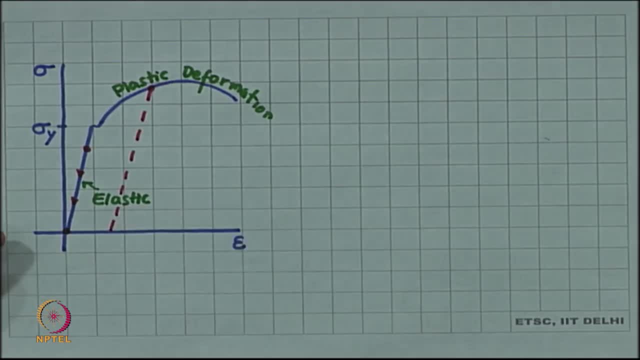 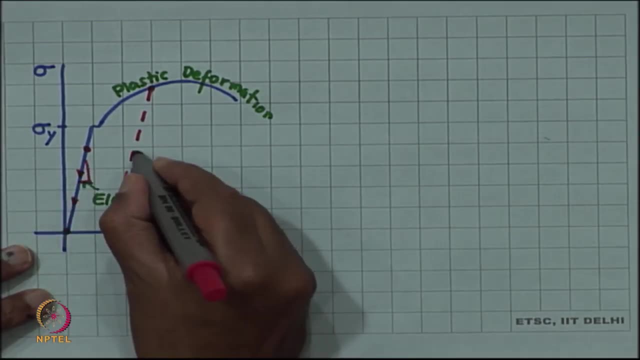 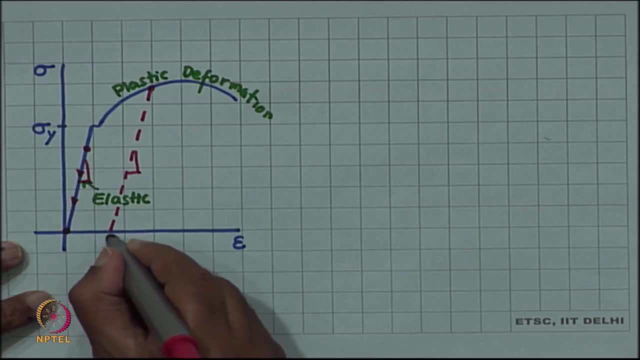 video. we saw the uniaxial tensile test and we saw that the initial part was in elastic deformation Parallel to the initial part of the curve. that is, the Young's modulus slope is not changed. that is the same, which means even at zero stress. so much of a strain. 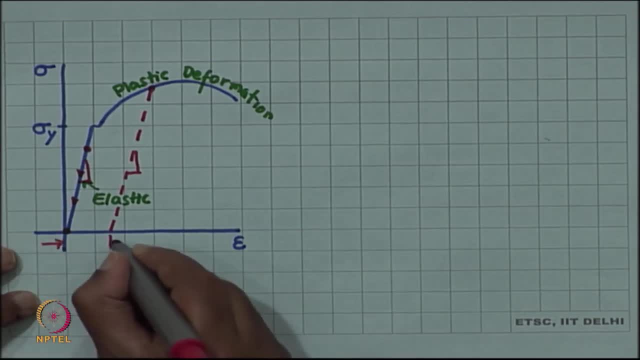 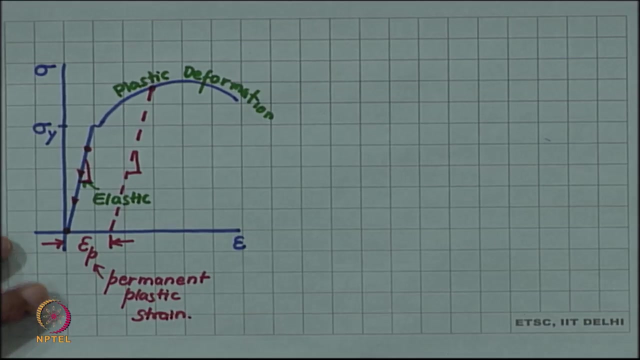 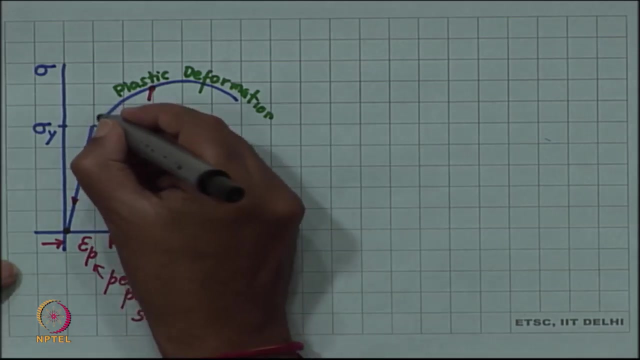 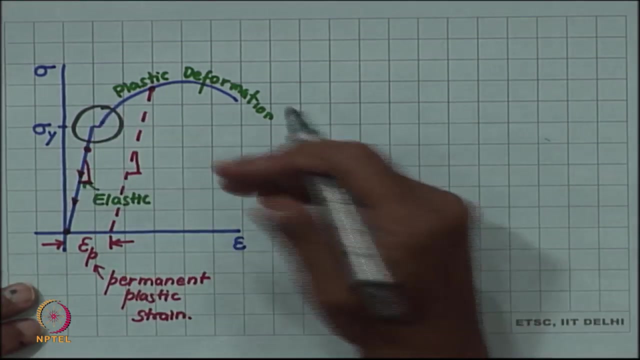 is left. So this is the plastic strain which is left in the material, Thank you, So let us focus on this part of the curve, the transition from elastic to plastic. So what really happens? What is in terms of the internal structure of the material, What really 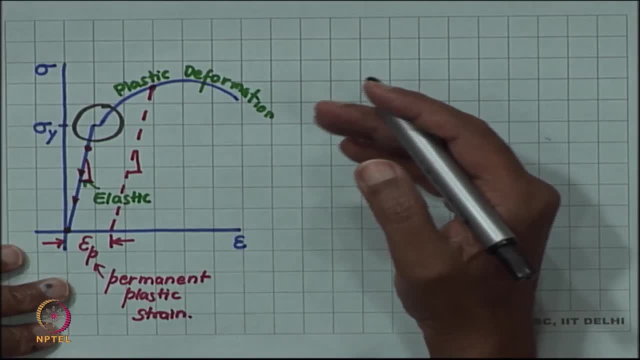 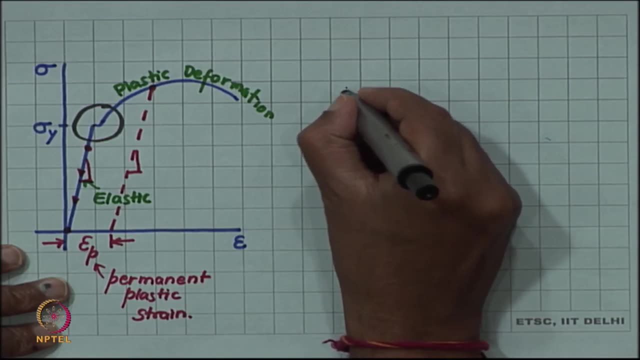 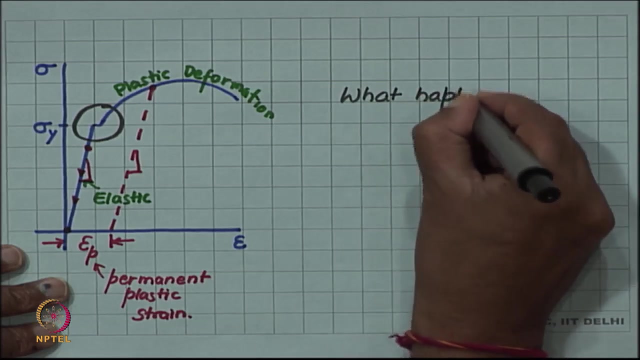 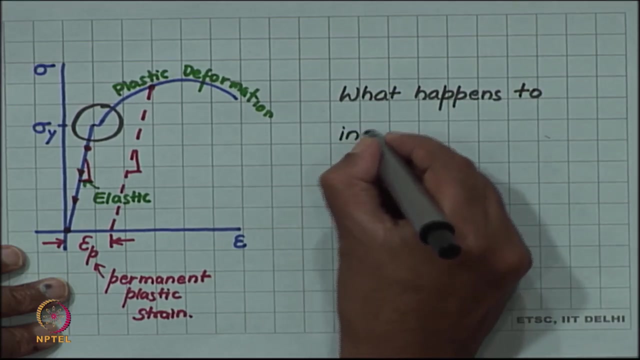 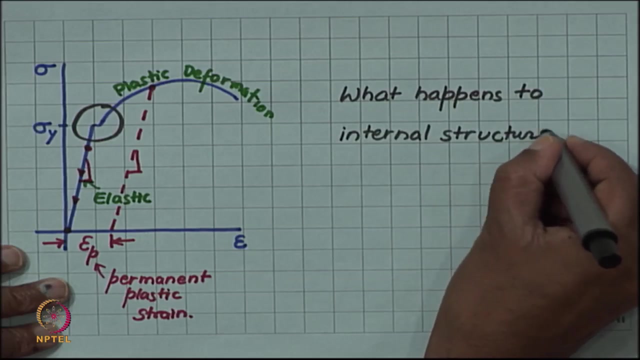 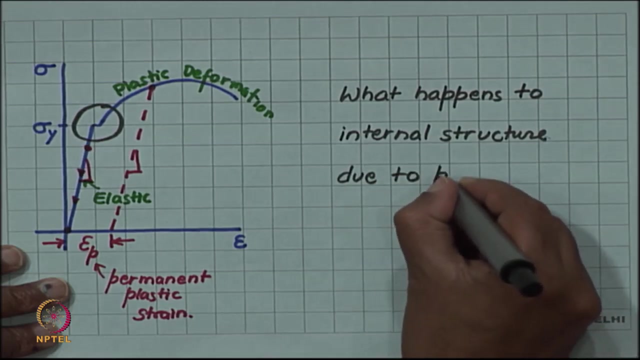 happens when it undergoes a transition from elastic to plastic deformation. So what happens? So what is the transition from elastic to internal structure? 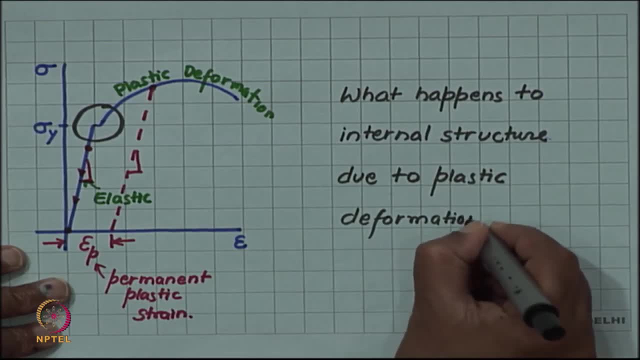 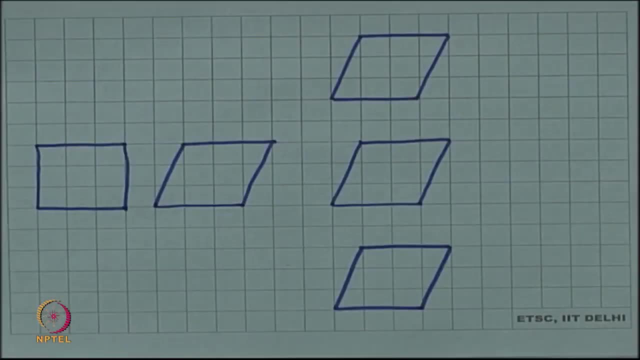 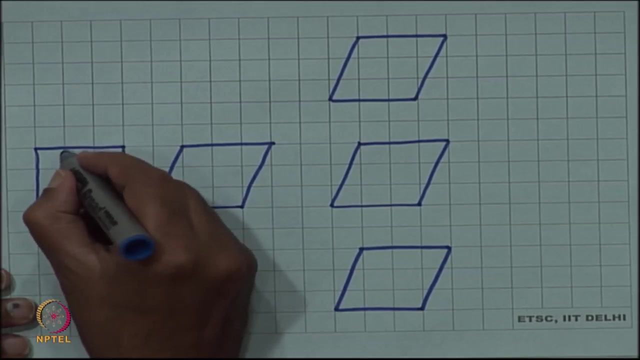 question little bit more precise. So let us think of that. we have a block I have shown you here in 2 D, but you can think of a 3 dimensional cubic block, and I am saying that. 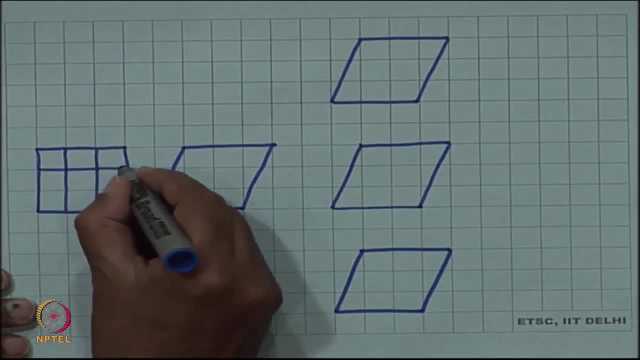 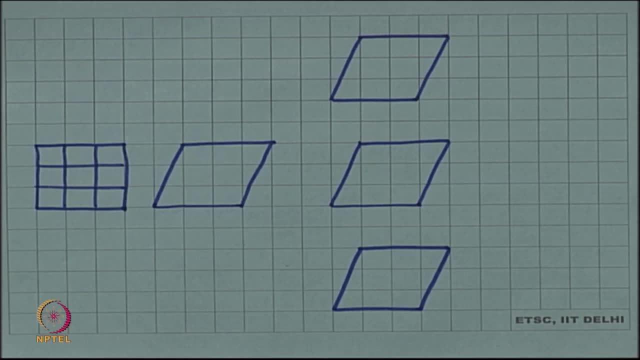 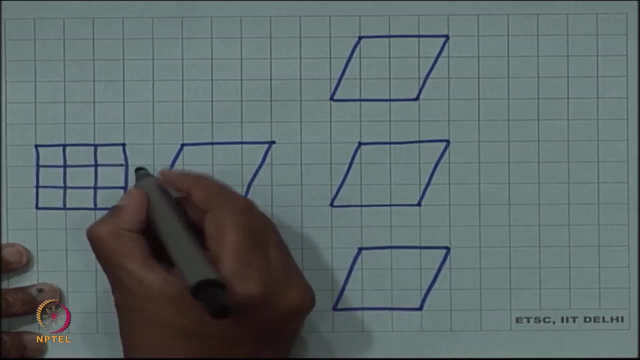 this material is crystalline. We know that most metals are crystalline. for example, copper is phase scented cubic. So the initial block which I am going to deform is crystalline. So by these squares I am trying to show some sort of crystal structure of this block. So 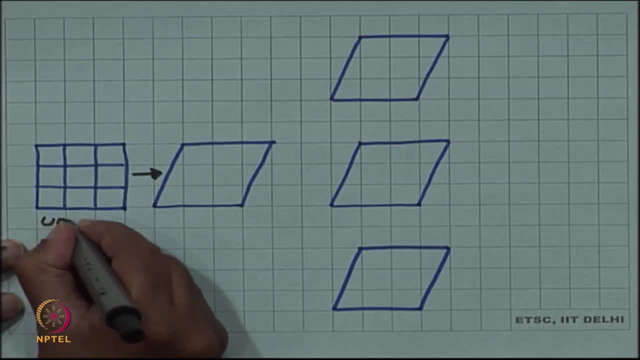 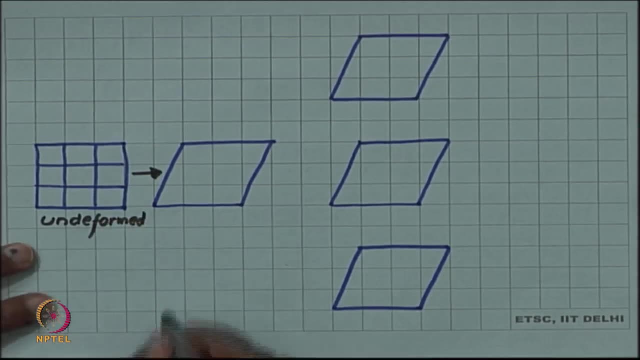 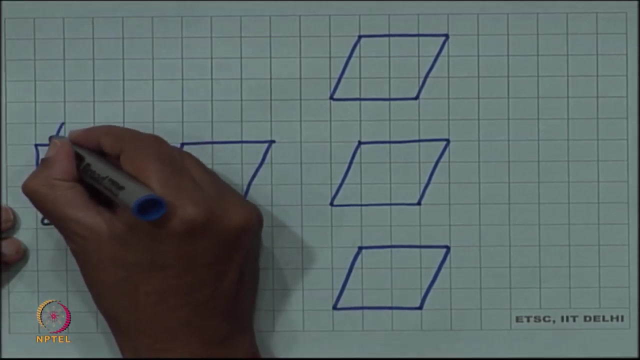 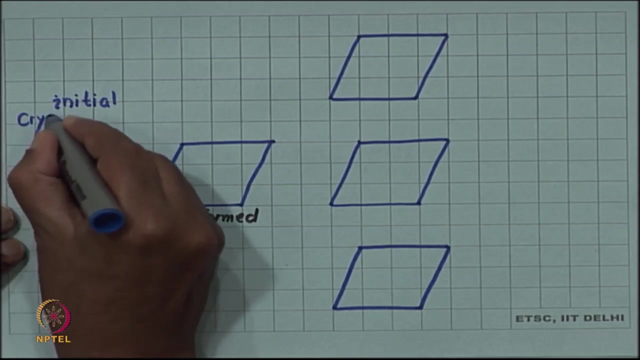 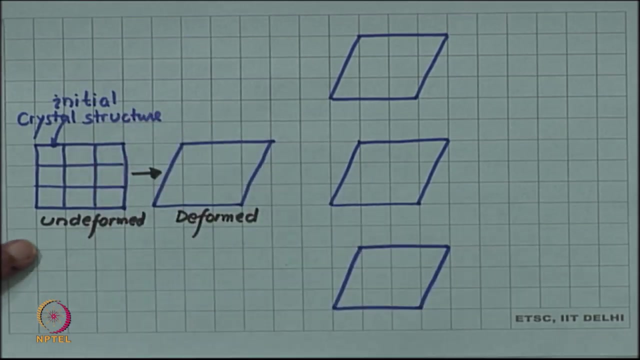 this is undeformed and now it is going to be deformed. So suppose it is deformed. now the question Which we are asking: what happened to the crystal structure? It had some initial crystal structure before deformation. The question is, what is the final crystal structure? So 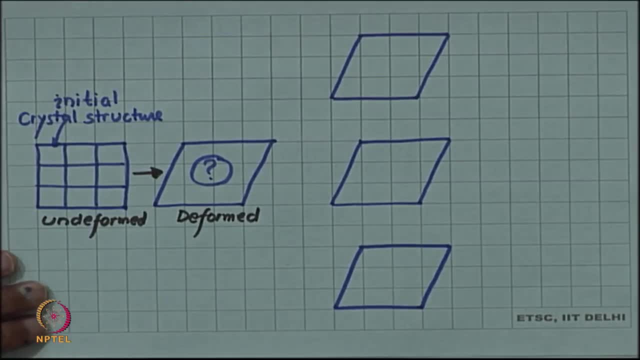 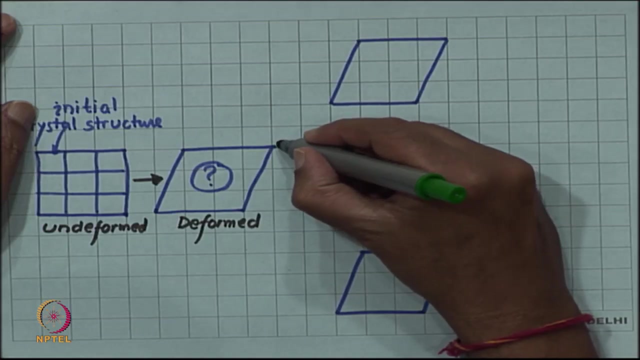 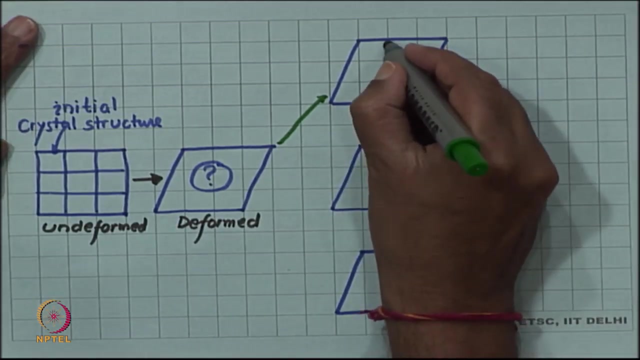 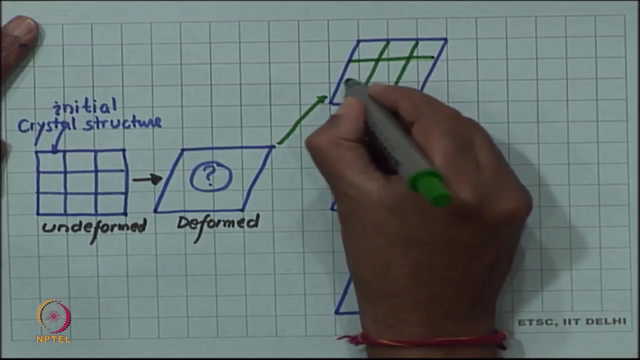 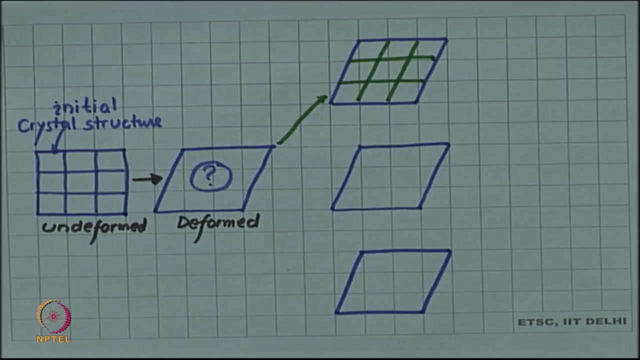 is it crystalline at all? Now, we can take several stands or several views about it. So one view could be that, as the material is deforming, the crystal structure also changes according to the deformation. This is quite natural to assume. So I think that the deformation has changed the crystal structure. Notice that in this. 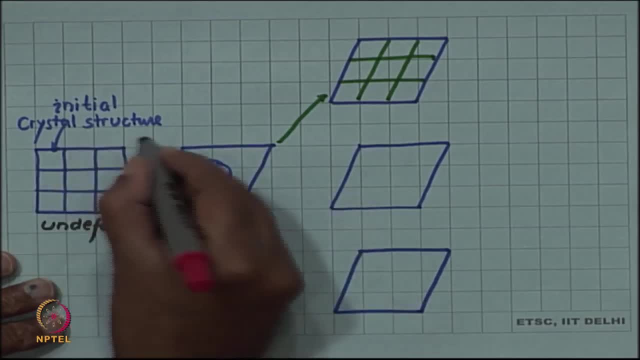 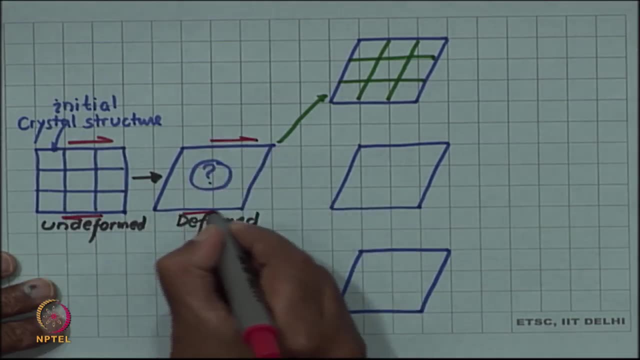 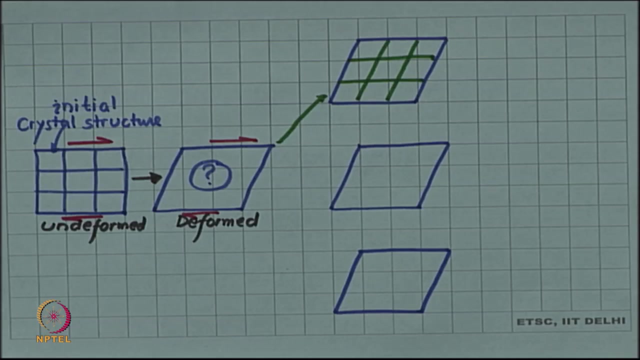 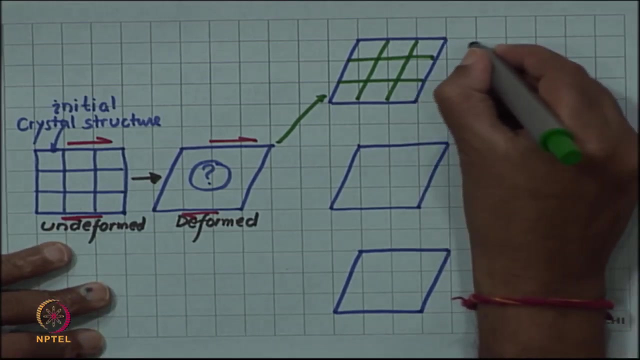 case I am considering a very simple kind of deformation, which is a shear kind of deformation Of the material. So one option can be: the crystal structure changes due to deformation, So this is the deformation of the material. So this is the deformation of the material. 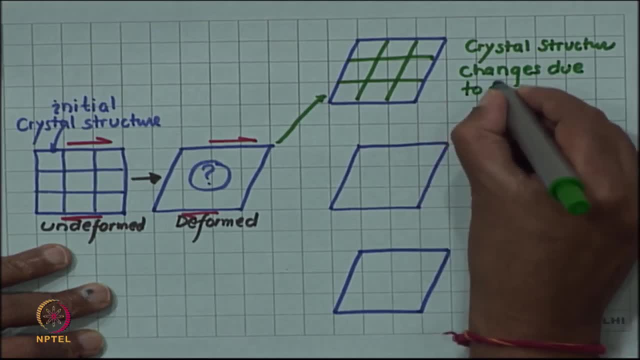 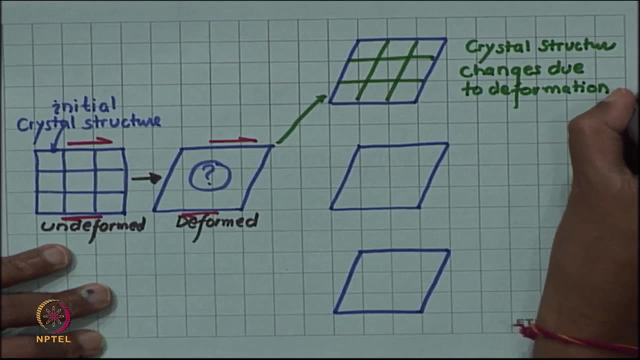 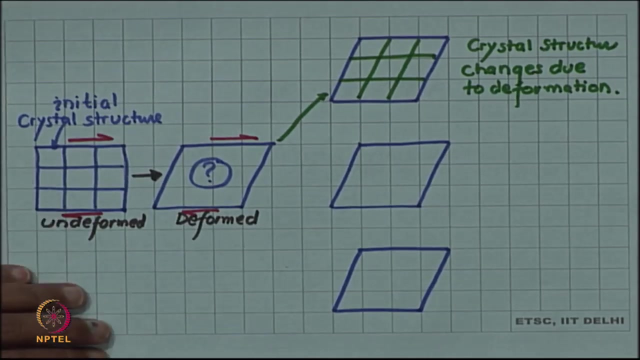 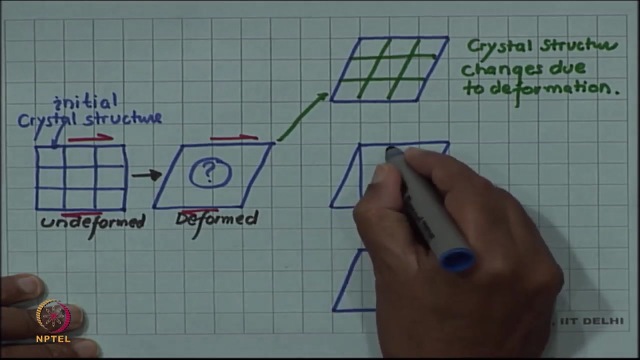 So this is the deformation of the material? I can take another view and I can say that no, the crystal structure is some sort of inherent material property and this does not change due to plastic deformation. The crystal structure remains intact. A given material will have a given crystal structure, irrespective of whether it is deformed or not. 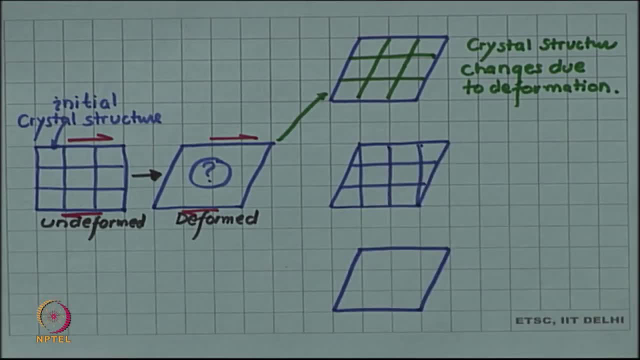 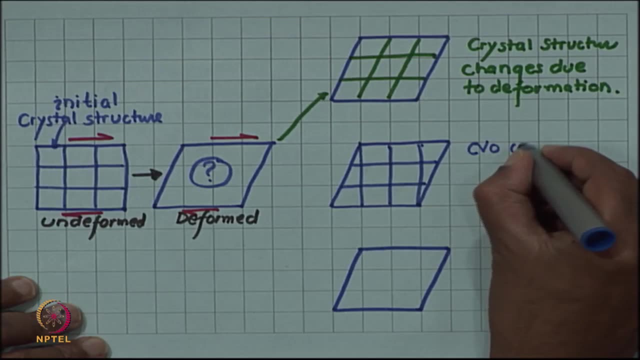 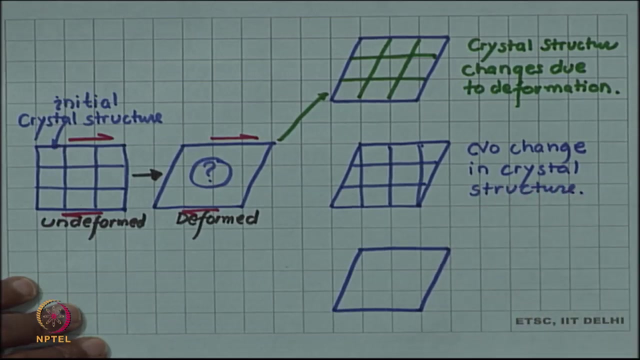 If I take this view and say that the crystal structure has not changed, So then I am saying no change in crystal structure- Yet another option we may think. we may think that the deformation can be quite aggressive in certain cases And due to deformation, due to plastic deformation, the material actually breaks down, the internal structure breaks down and the crystal structure is lost. 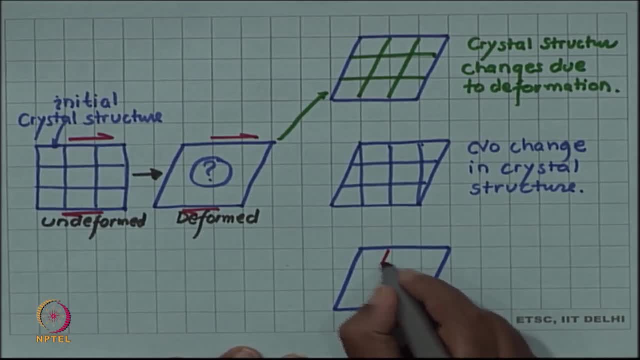 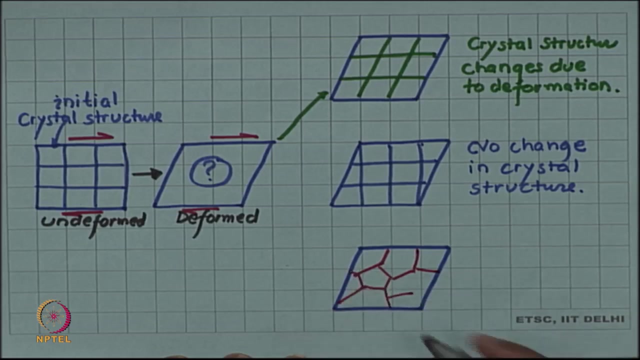 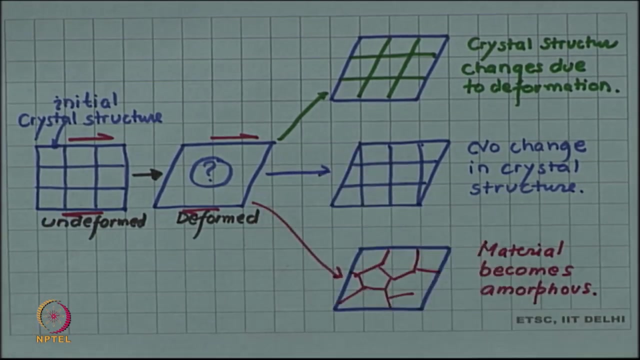 So So It sort of becomes. I am drawing this to just to show that the unit cell has broken down and some sort of amorphous structure has evolved. so no crystal structure is left, material becomes amorphous. I have given you these three options. you may even think of yet another, some other new. 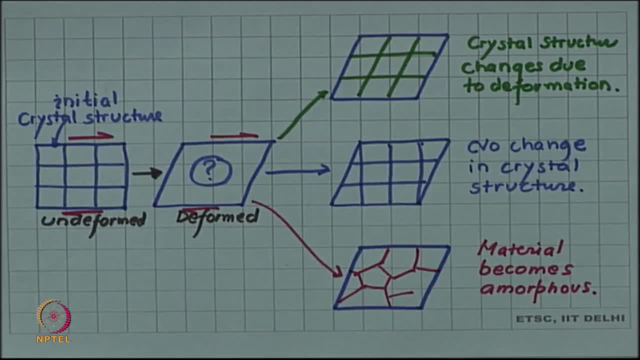 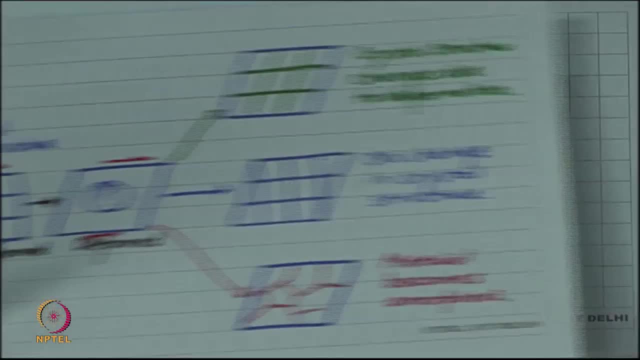 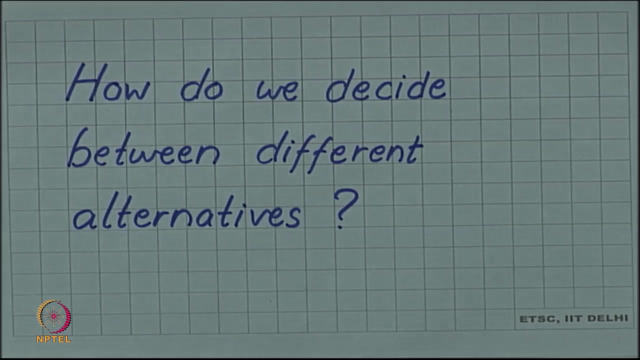 option Rather than these three. but the question is: how do we decide? How do we decide between these three alternatives or any other alternative that you think of? What is the basis for decision? How do we say whether the crystal structure changes or does not change, or the material? 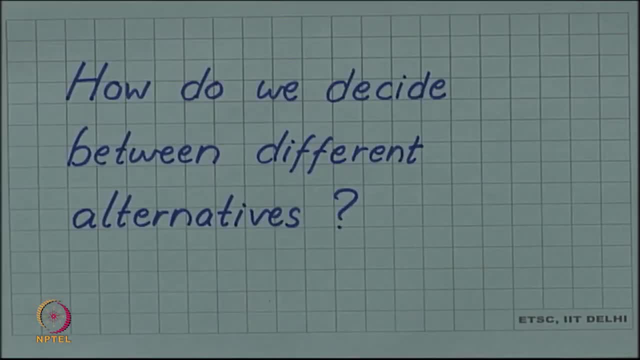 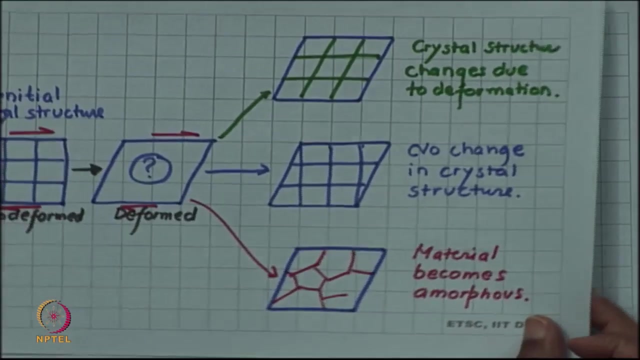 becomes amorphous. So how do we decide between these different alternatives? This is where a great scientific, Great distinction comes from the ancient scientists like Aristotle. so Aristotelian thinking would have been to just by pure thinking, decide which of these three alternatives appears. 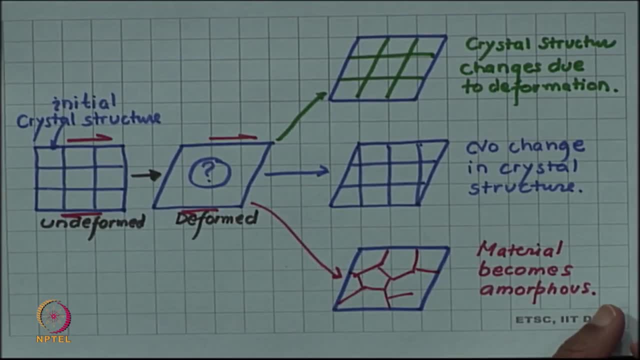 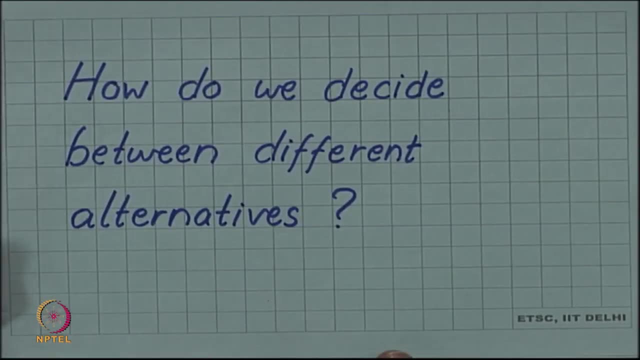 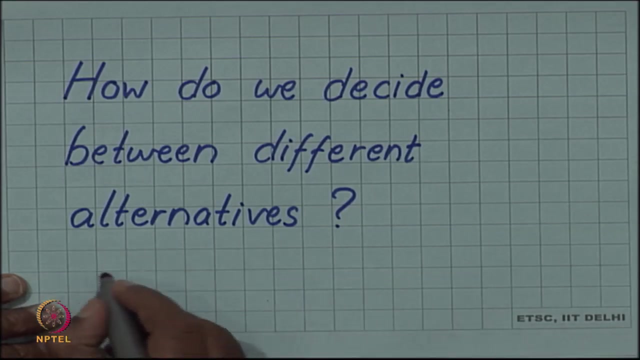 to be right or logically consistent with previously known knowledge. But in the modern science we let the nature decide the question. and to let the nature decide we do experiments. So we will have to do experiments. So the correct way to decide between the alternatives is experiment. 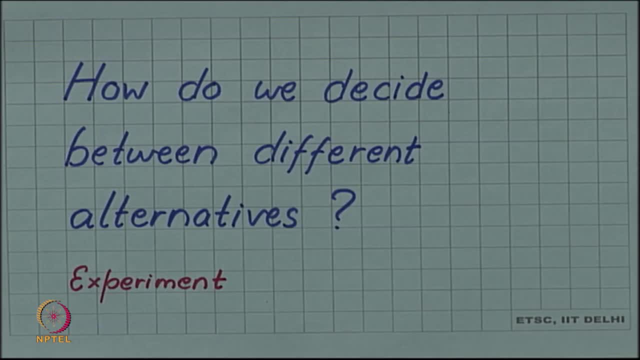 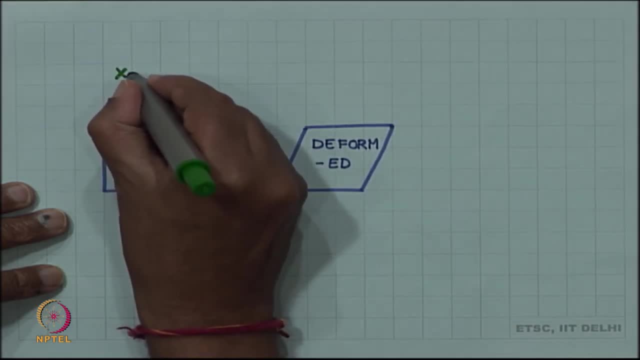 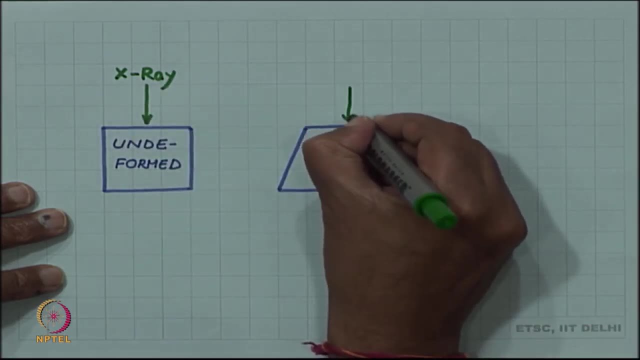 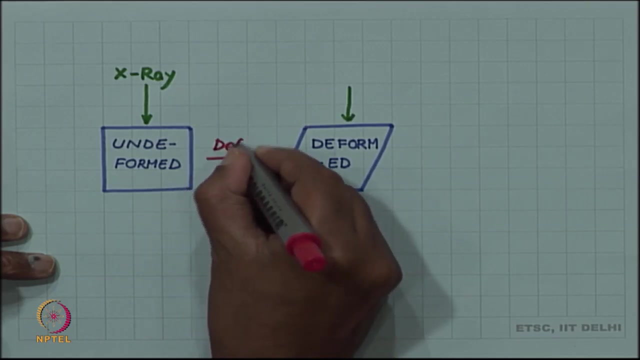 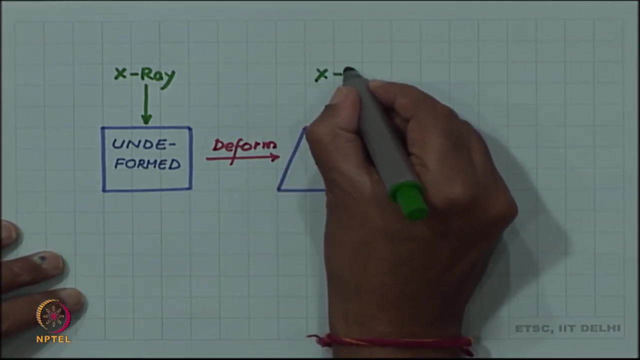 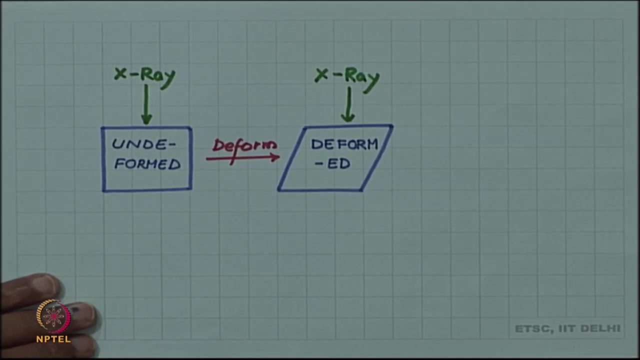 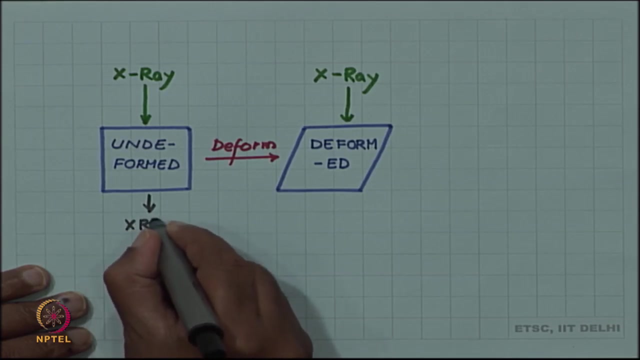 x ray on undeformed material and I also sign and then I deform it and I do the experiment again. I sign x ray on the deformed sample. Both will give me diffraction pattern, x ray diffraction, and when we analyze the diffraction pattern we can solve the problem.